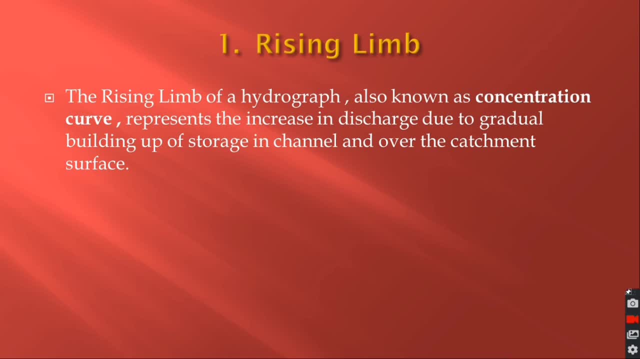 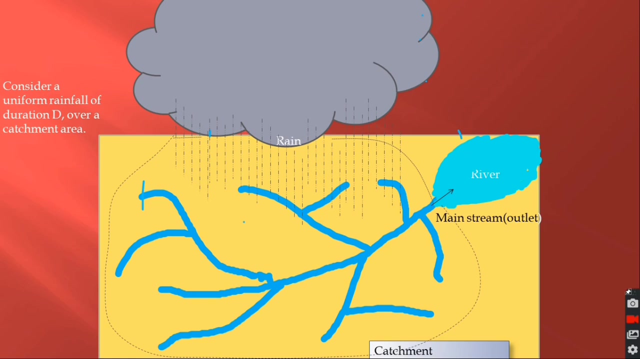 curve represents the increase in discharge due to gradual building up of storage in canal and over the catchment surface. this was catchment area over which rainfall for duration D occurred. we have seen, after the initial losses of water through infiltration, interception, evaporation, etc. water collect on the catchment surface and in the canals and 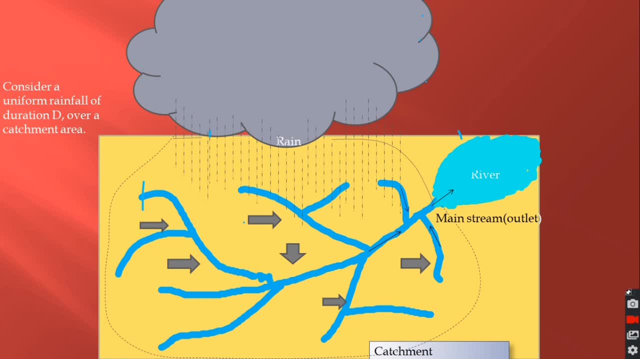 then this water began to run off towards catchment outlet. this area, which is nearest to outlet of catchment, runoff will from here first, this one, after that area which is away from outlet. runoff will occur from there, from this part, and, like this, water will begin to runoff from different areas and, at last, runoff. 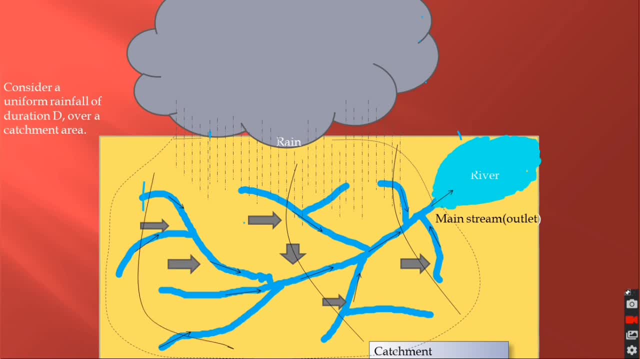 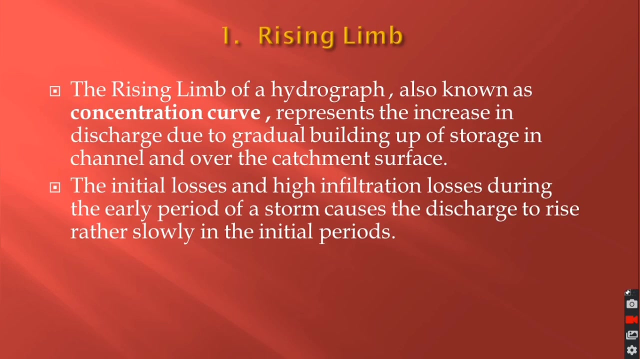 will occur from remotest area this farthest part. so that is why the discharge at the outlet will increase with time. the initial loss and high infiltration loss during the early period of storm caused the discharge to rise rather slowly in the initial period. the rising limb will increase slowly in initial period due to losses we have. 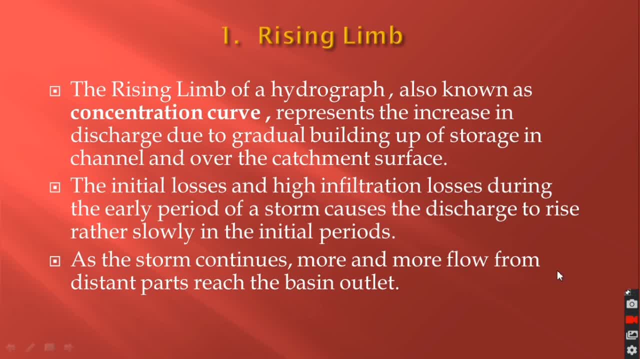 discussed that and as the strong continues, more and more flow from distant part reach the basin, outlet basin and strong characteristics control the shape of rising limb. means rising limb will depend on basin or watershed characteristic, such as so that ah, the cleavage in kinderen that is the base of the고요 areas, or down onto distant areas. 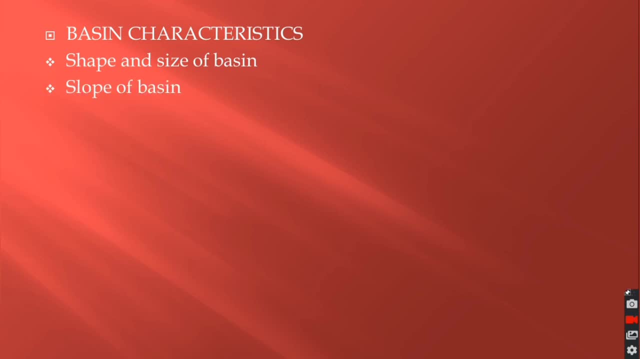 shape and size of basin, slope of basin, drainage, density, etc. for example, if basins shape is elongated or fun shaped, like this, rising limb will increase slowly and the peak of hydrograph will be low. if basins shape is fan shaped, that is, nearly circular shape like this, then in this case rising limb will increase. 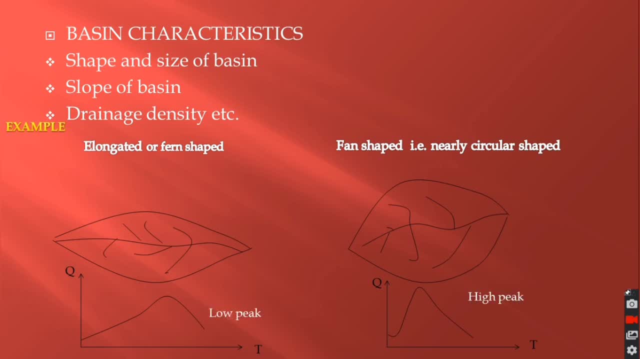 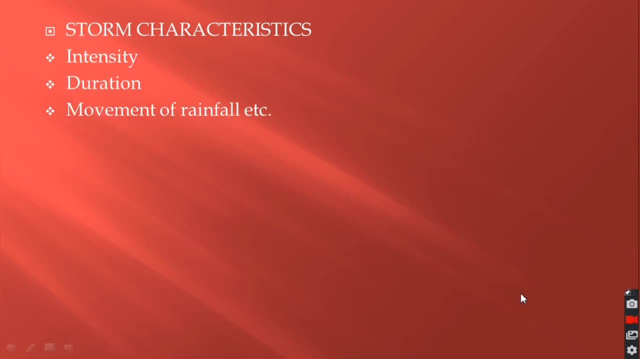 rapidly and the peak of hydrograph will be high. rising limb will also depends on the strong characteristics such as rainfall intensity, duration, movement, etc. this was all about rising limb. now let us see about crest, or peak segment. this is important part of our graph as it contains peak flow. 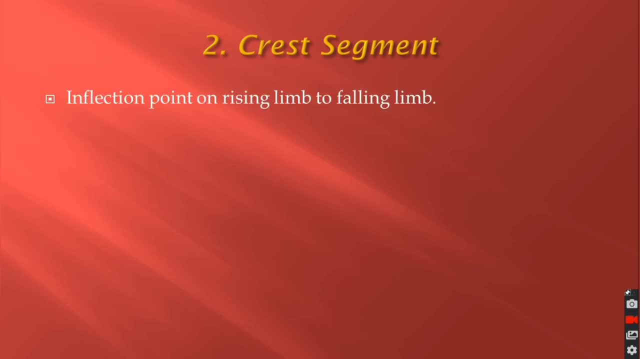 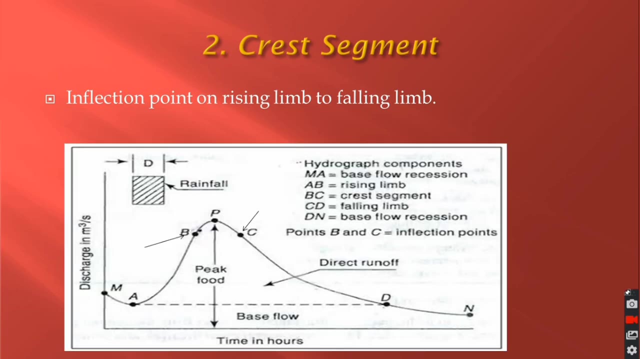 crest segment is from inflection point on rising limb to falling limb. point B and C are inflection point. inflection point is the point where curvature of the curve changes. as you can see, up to the point B curve was something concave and after that it became convex. from point B to C. 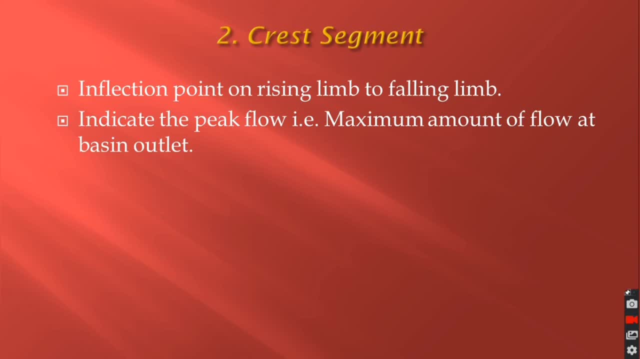 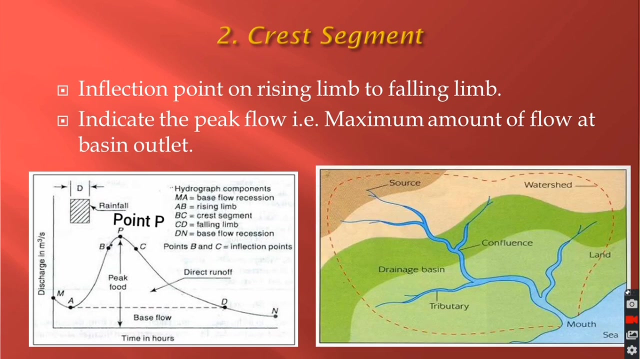 crest segment indicate the peak flow, that is, maximum amount of flow at basin outlet. maximum amount of flow is obtained at point B and it generally occurs when the runoff begin to occur from farthest area of catchment. the peak flow occurs when runoff various part of catchment simultaneously contribute. 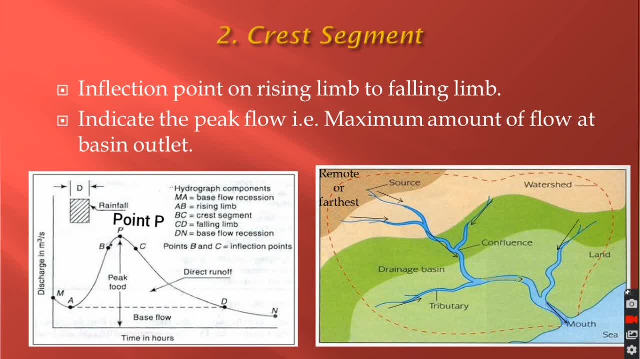 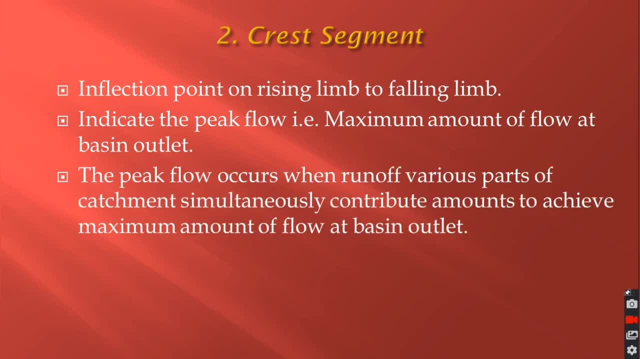 amount up to achieve maximum amount of flow at basin outlet. this is only written here and generally for large catchment peak flow occurs after cessation of rainfall means in large catchment peak flow of occurs after rainfall stop, as it will take time for the runoff to move from different part of. 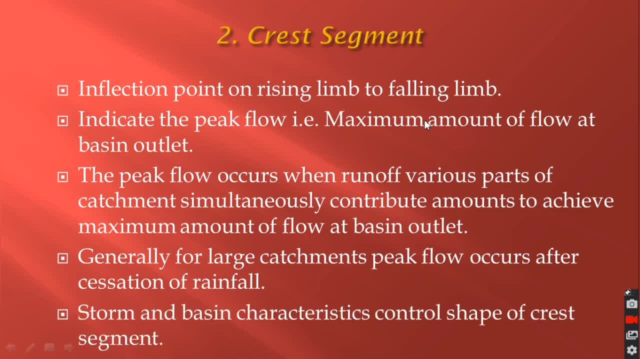 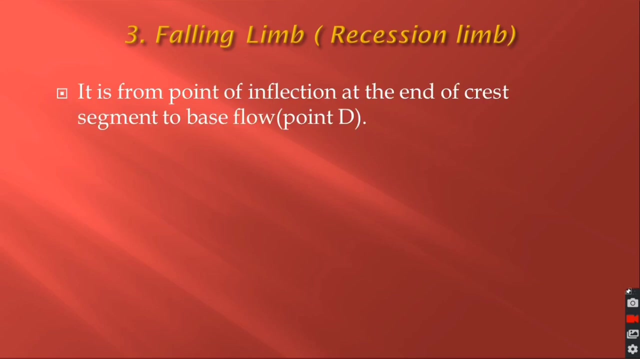 catchment, storm and basin characteristics control. shape of crest segment means the shape of crest segment, like rising limb, also depends on basin and strong characteristics. now let us move to falling or recession limb. it is from point of inflection at the end of crest segment to base flow, point d. 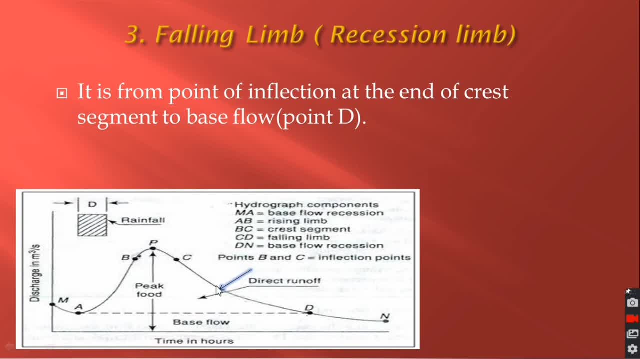 means from point c to d, inflection point represent the time at which rain stop. that is condition of maximum storage. when rainfall will stop, at the time storage of water will be maximum and after that storage will begin to deplete due to runoff at the basin outlet. 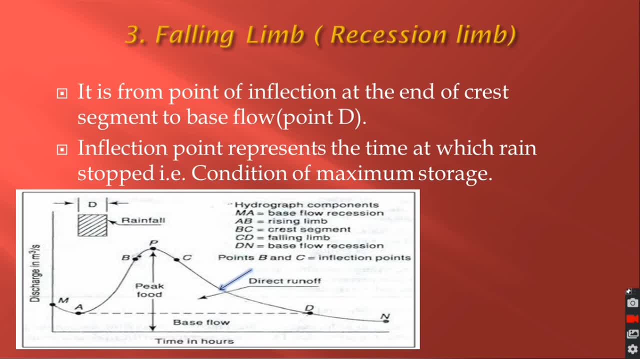 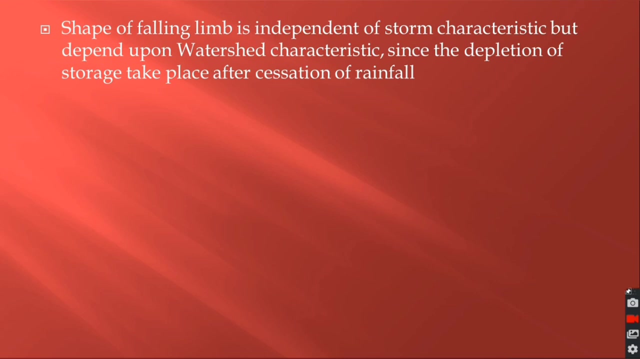 and the hydrograph slope will fall or decrease. that is the thing it's saying. point c is the point when rain stopped and it is a condition of maximum storage. shape of falling limb is independent on storm characteristic but depends upon watershed characteristic, since the depletion of storage take place aftereking of rainfall. 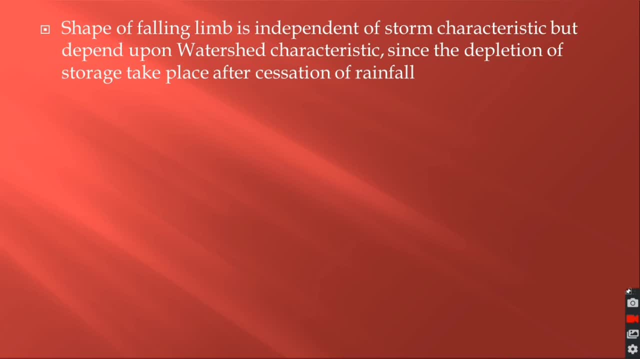 after the rainfall stop. So it only depends on watershed characteristics. Obviously, when there will be no rainfall, how it will depend on storm characteristics. Rising limb and crest segment were dependent on storm characteristics, But falling limb will not depend. So these three were important region of hydrograph. I hope you all understood it. 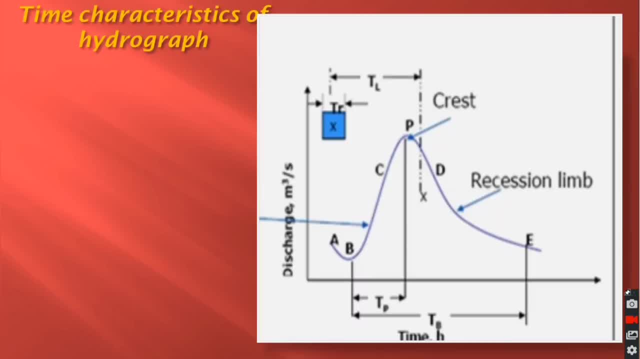 Now let's see about time. characteristic of hydrograph. First is time base of hydrograph. You can see in the picture. This is the time base from B to E. This is the time base from B to E. This is the time base from B to E. 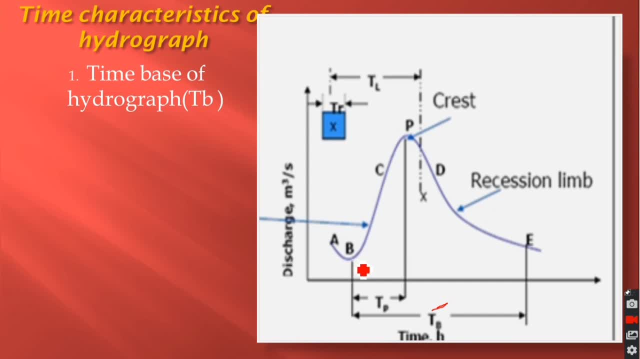 B is the starting point of direct runoff, Means when the surface runoff started, And E is the end point of direct runoff. Below the direct runoff we have base flow Means- initial groundwater flow of stream or canals. This is the time base of hydrograph. 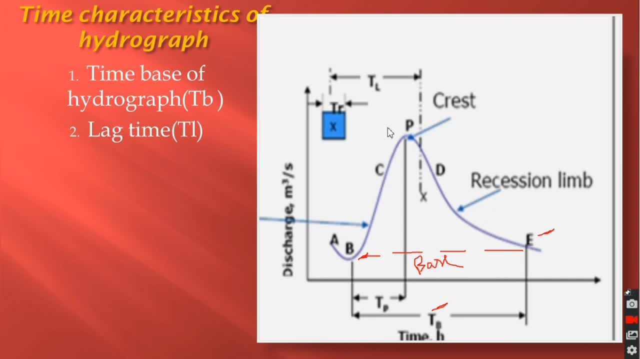 Second one is lag time T L. Here it is, From centre of mass of rainfall to centre of mass of hydrograph. And the third one is time to peak Here, from point B, That is starting to direct runoff, to peak flow point P. and fourth, rainfall duration. Here it is. It shows the duration for which rainfall 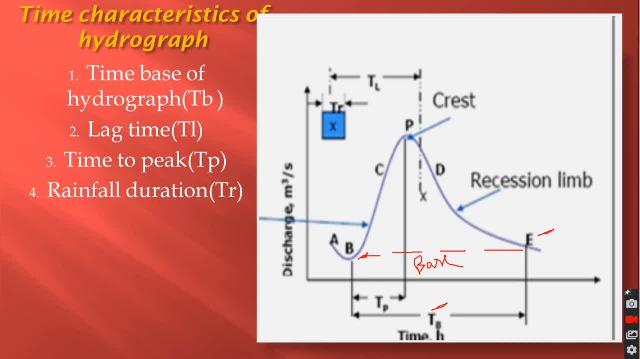 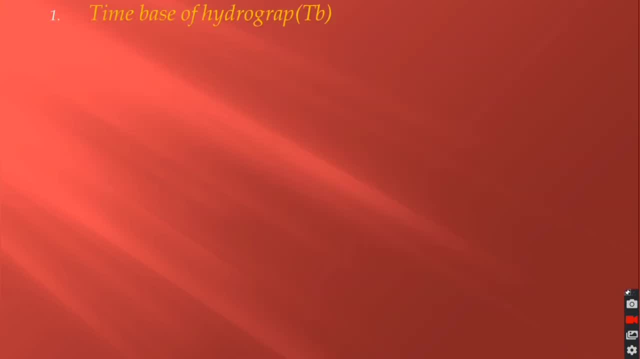 occurred. So let's look the definition of this Time base of hydrograph. It is the time from beginning to end of direct runoff, From point B to point E. That is beginning and end of direct runoff. Lag time, It is difference. 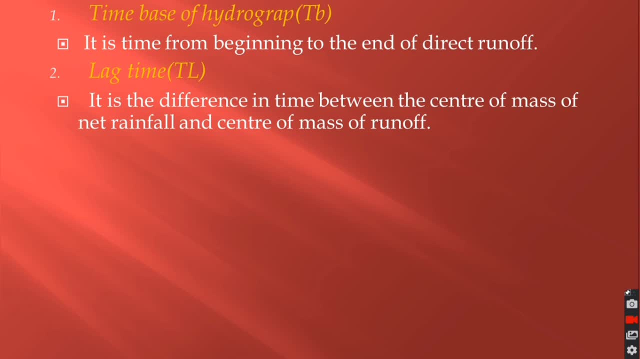 in time between the centre of mass of net rainfall and centre of mass of runoff Means time between maximum rainfall and maximum runoff. Third one is time to peak. It is the time difference between the beginning of direct runoff, point B, to peak- We saw it. And fourth one: rainfall duration. It is the effective. 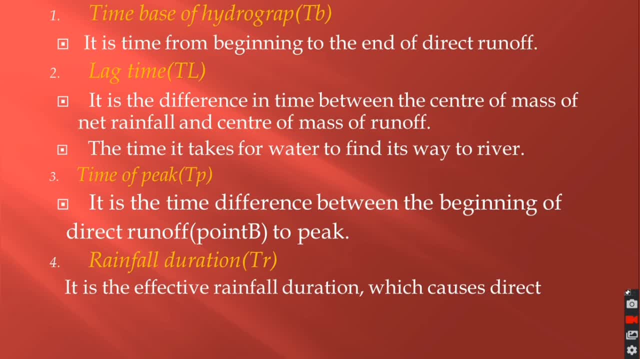 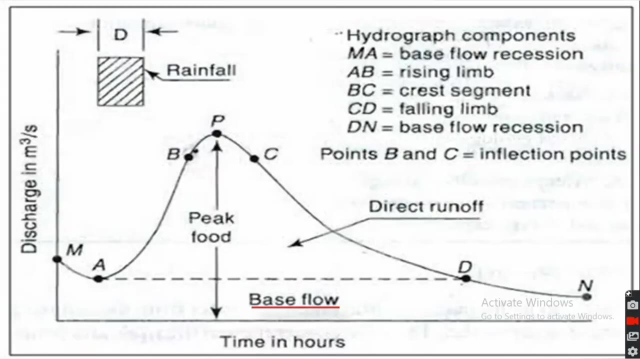 rainfall duration Which cause direct runoff. This was all about time. Characteristics of hydrograph. Now let's see what is base flow, direct runoff and interflow terms in hydrograph. First base flow is normal discharge of the river. First base flow is normal discharge of the river. 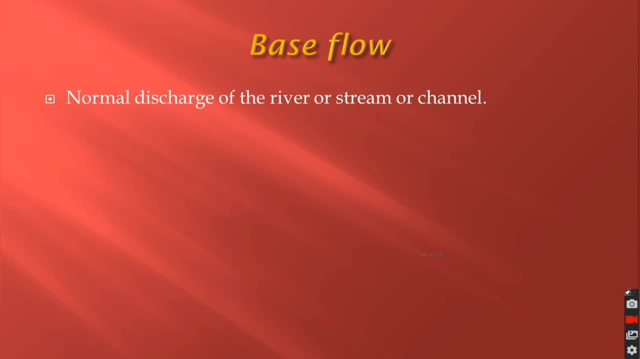 First base flow is normal discharge of the river. Second base flow is normal discharge of the river or stream or canal. It means before rainfall there must be some ground water table flow. This ground water flow is called base flow Suppose. this is a side view of a catchment. 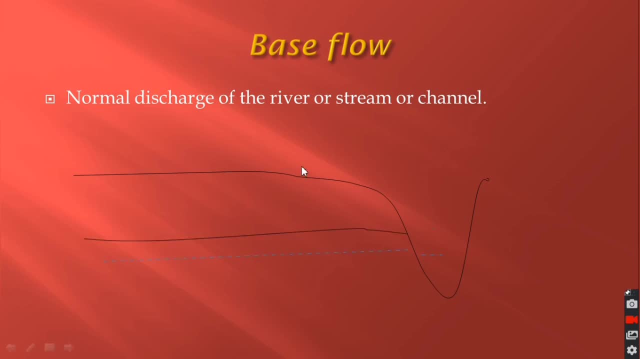 This is the surface and this is the ground water table below the surface of catchment catchment. when rainfall will occur, some water will infiltrate through the rocks and pebbles and delaying the surface, and some water will run off to streams from the surface. 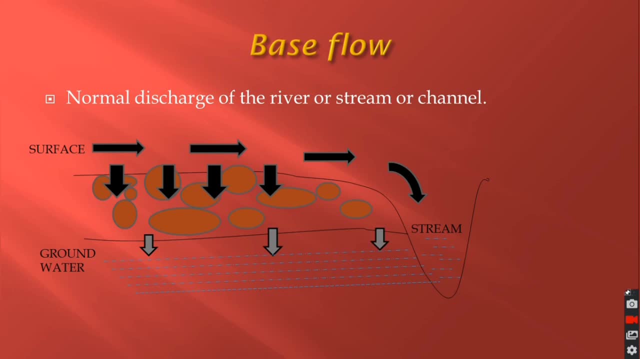 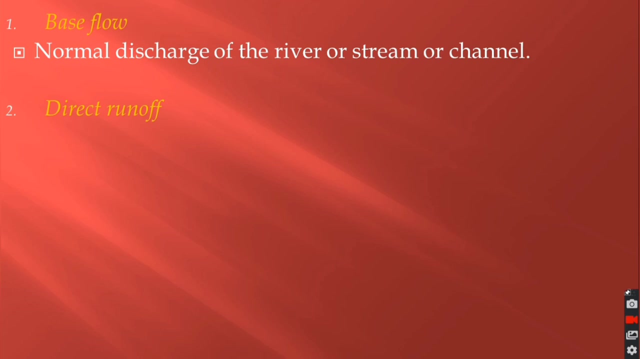 after infiltration, some water will reach the groundwater table and this ground water will reach to the stream and will discharge. this is called base flow and the runoff above the surface is called direct runoff. direct runoff volume of water reaching the river outlet from the surface runoff and inter flow volume. 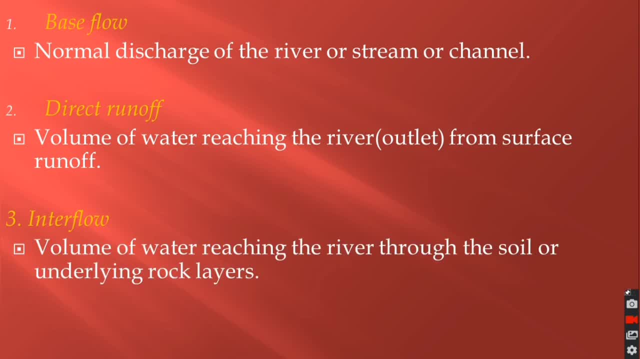 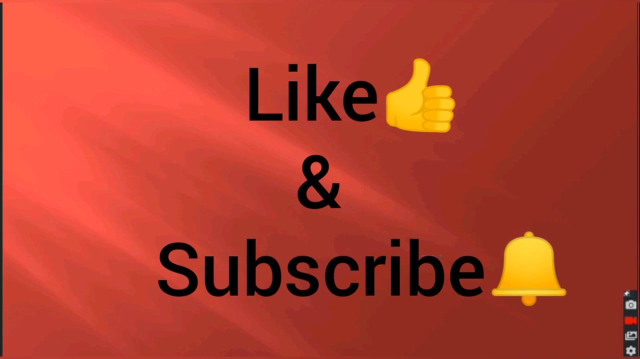 aniu of water reaching the river through the soil or undulating rocks layer. as we discussed earlier, hydrograph consists of flow in all these three phases of runoff. all the, all these three runoff will be seen in hydrograph. please like and subscribe our channel, and press the bell icon for more updates.